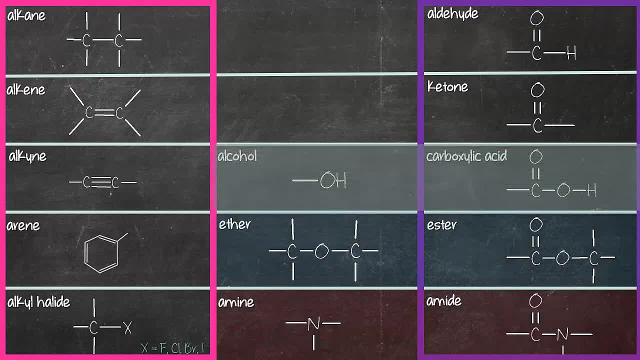 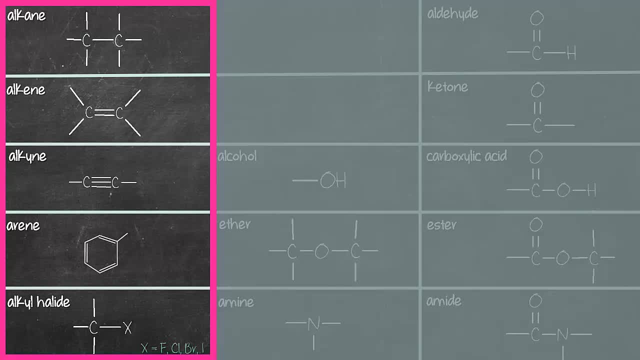 For each of these groupings. let's look at the first grouping. They are all hydrocarbons, except for the fifth one, alkyl halide. It's a hydrocarbon derivatives. Hydrocarbons are compounds that consist of only carbons and hydrogens. So let's focus on the first three: alkane, alkene and alkyne. 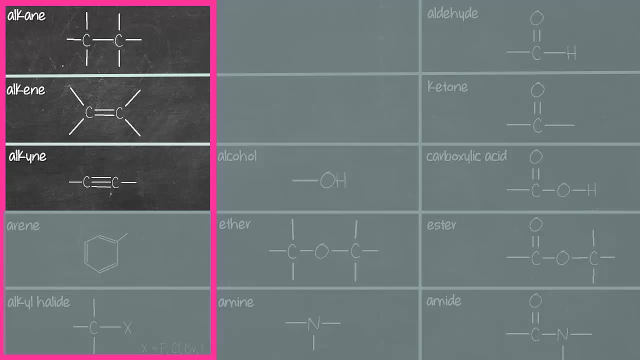 These three are quite similar aside from the spelling. They are the triplets. They differ only by one alphabet: A for alkane, E for alkene and Y for alkyne. So think of it this way: A comes before E, E comes before Y. 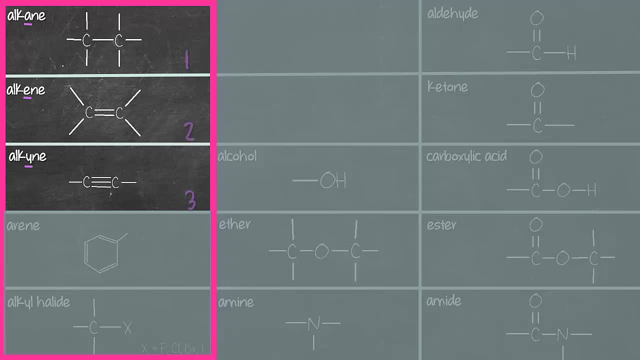 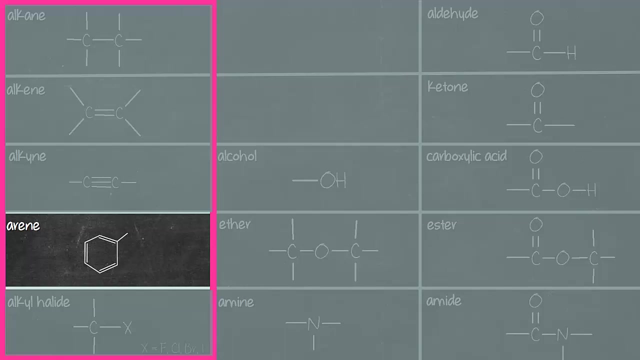 So the number of bonds between the C and the C, it's single bond in alkane, double bond in alkene and triple bond in alkyne. A, E, Y, 1,, 2,, 3.. Next we have arene, which is also called an aromatic group At introductory chemistry level. 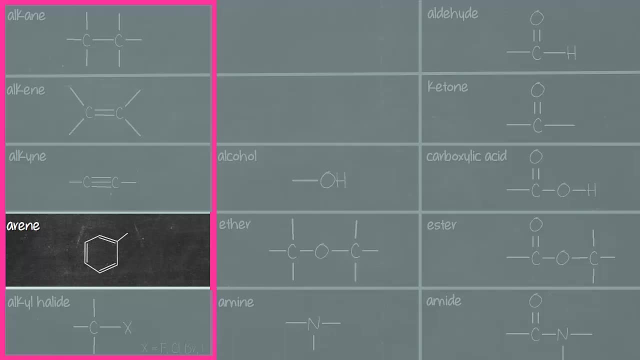 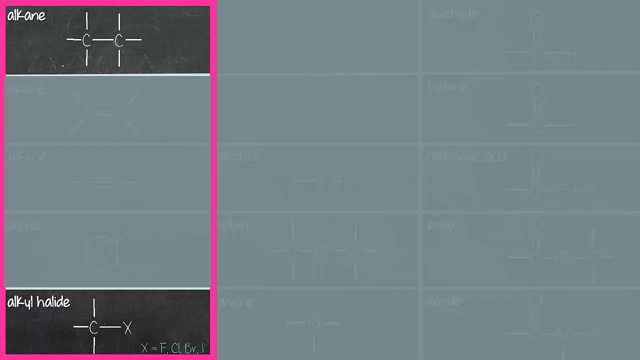 the arene you will encounter will be benzene ring, which consists of six carbons with alternating single and double bonds. Then we have alkyl halide, which is the hydrocarbon derivatives. It's actually an alkane, except for it's missing one hydrogen, and that's replaced with a halogen, like fluorine, chlorine, bromine and iodine. 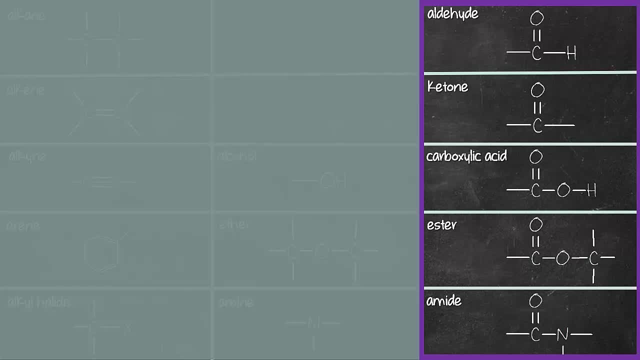 Moving on to the next grouping, what do these guys have in common? It's that C double bond over here They are actually called carbonyl. If you attach OH next to a carbonyl group, then you get yourself a carboxyl group. 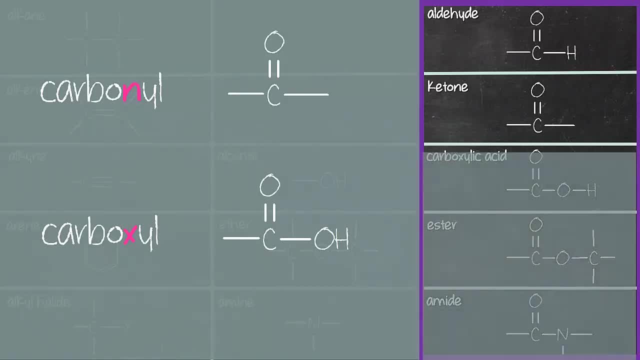 The difference is only N and X. So what's the difference between aldehyde and ketone? Look closely between aldehyde and ketone. They both have C double bond O. The difference is that aldehyde has a hydrogen right next to that C double bond O, whereas ketone 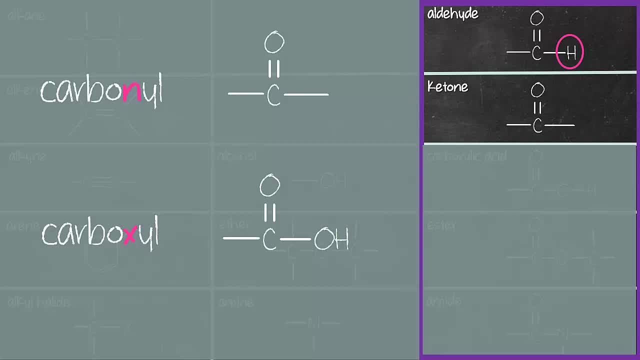 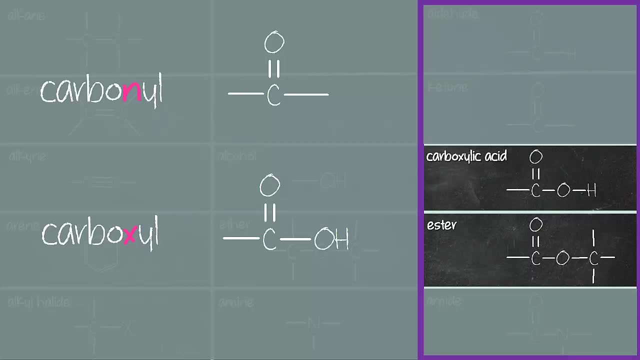 on the left and on the right. on both sides of that carbonyl group are going to be carbons. Next we have carboxylic acid and ester. What's the difference between these two? Well, the difference is that carboxyl group is present in carboxylic acid. 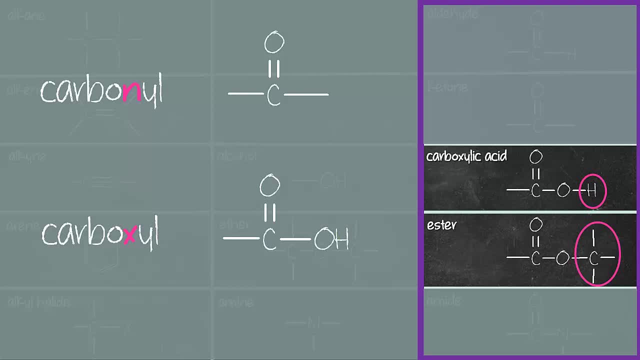 and that H in carboxylic acid is replaced with a C in ester. So functional group for carboxylic acid is COOH. Functional group for ester is C, So functional group for carboxylic acid is C. double bond O- OC. 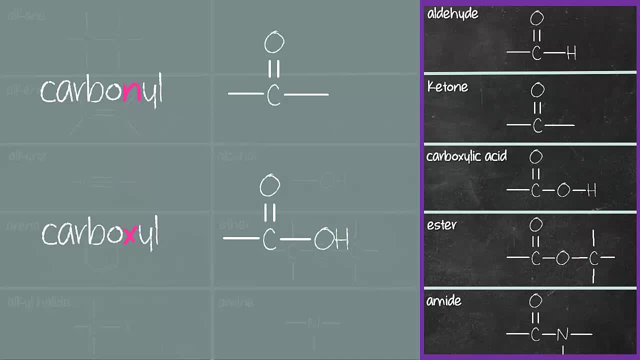 And last, in that group that also has C double bond O is amide. The difference between amide and the rest is that, aside from that C double bond O, next to it is attached to a nitrogen which has three bonds. So that's the difference between all of these carbonyl groups. 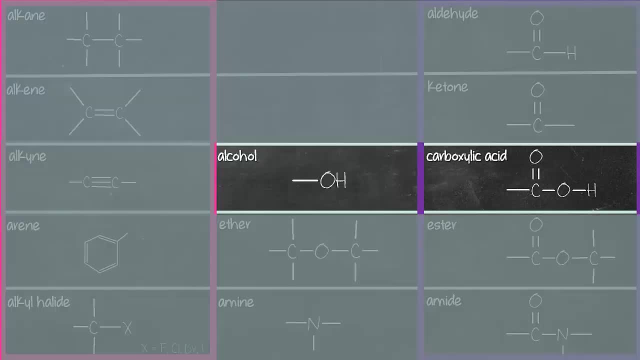 Okay, next we move on to the next grouping: alcohol and carboxylic acid. Now they are both. they both have something in common, which is the OHase. OHase is the OHase group, which is the OHase group, which is the OHase group. 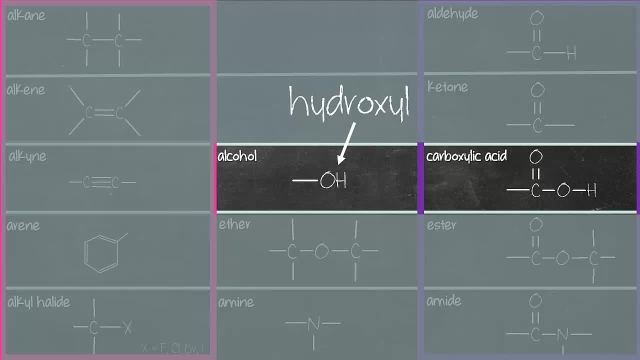 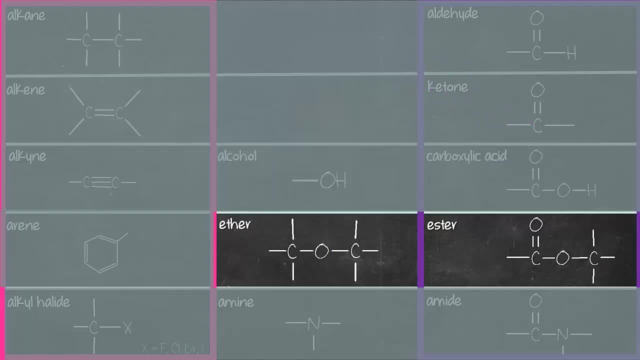 By the way, OHase group has its own name. it's called hydroxyl group. So if you look at the difference between alcohol and carboxylic acid, they both have OH. The only difference is carboxylic acid has an extra C, double bond O. 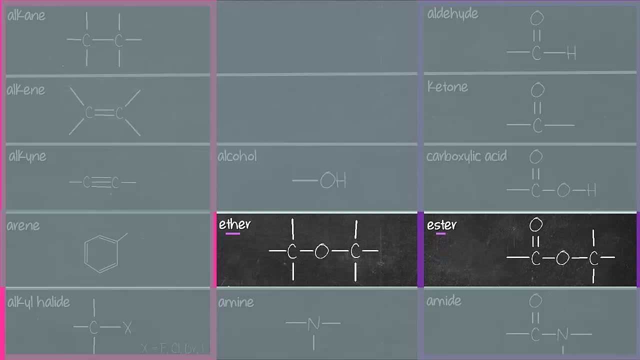 Next we look at ether and ester. Ether and ester are spelled quite similar so don't get confused. Ether is E-T-H-E-R. Both birds are different so don't get confused. But they're kind of similar like alcohol and carboxylic acid. 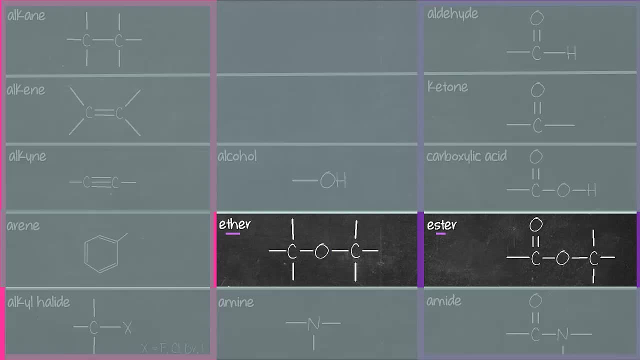 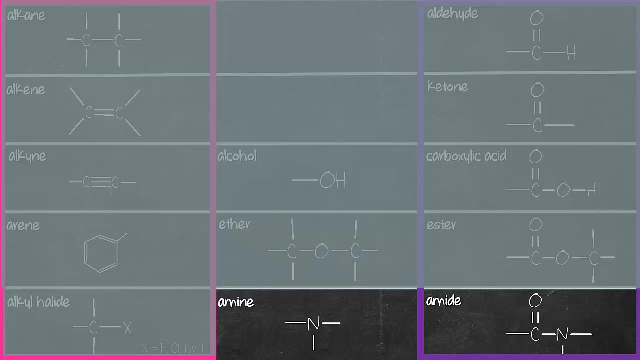 So these two, they have carbon, oxygen, carbon right in both sides, But if you look at ester, one of that C is actually a carbonyl group. So that's the difference between these two. Last but not least, we look at our nitrogen compound, which is amine and amide. 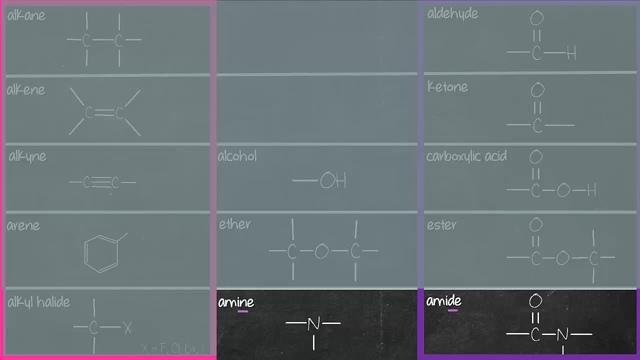 So they are also spelled quite similarly. So the difference between the spelling is: amine is spelled with an N, amide is spelled with a D, And the difference between the two, in terms of their functional group, is that amide has a carbonyl group. 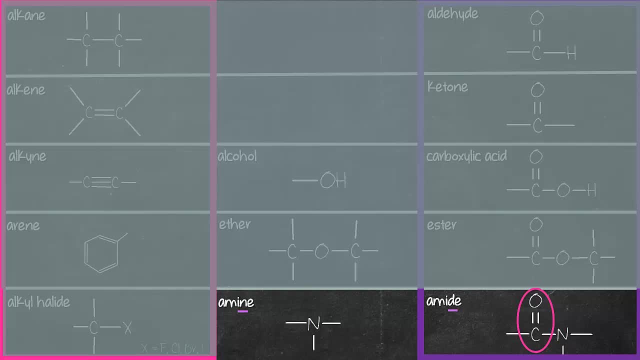 Whereas amine doesn't have a carbonyl group. They both have nitrogen, which has three single bonds, But in amide there's a carbonyl group right next to that nitrogen. And that ends the intro to the 13th lesson.